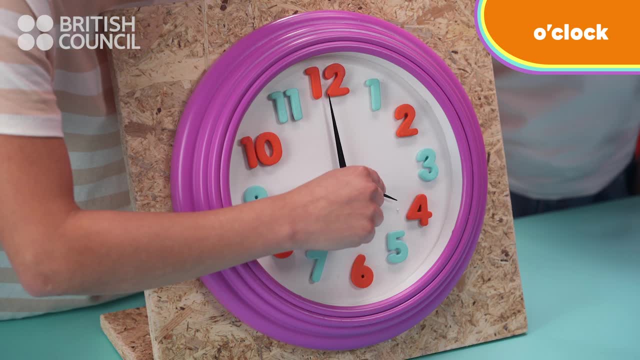 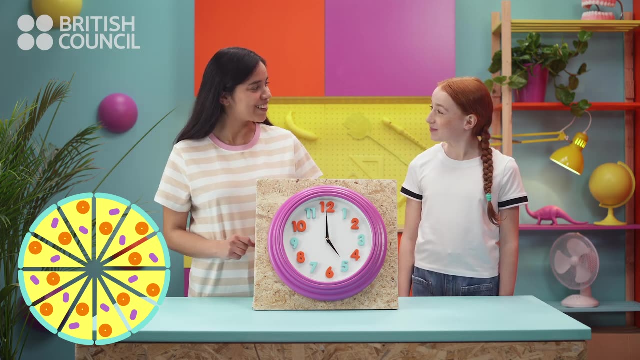 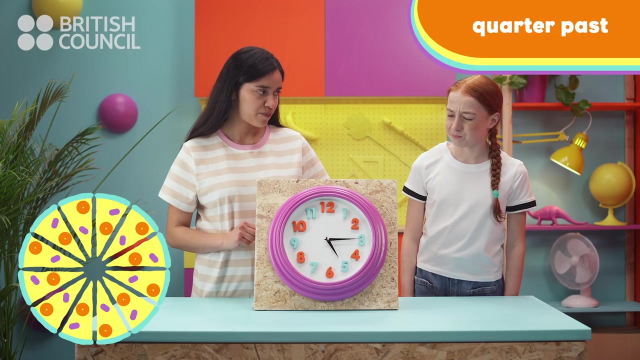 Now it's 4 o'clock. So, Emily, what's the time now? Now it's 5. 5 o'clock, Very good. When the big hand is pointing to the 3, we say it's quarter past. Mmm, why do we say it's quarter past? 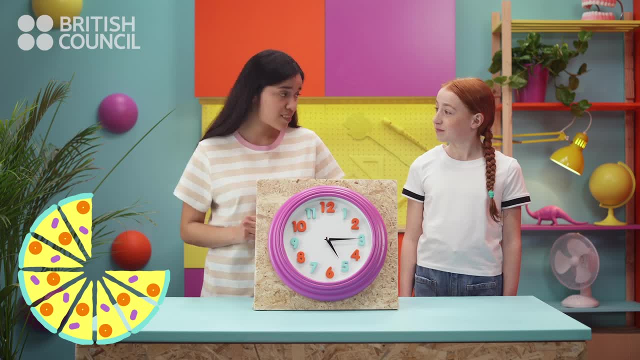 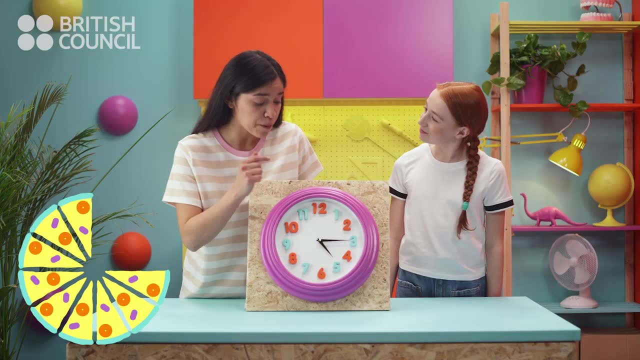 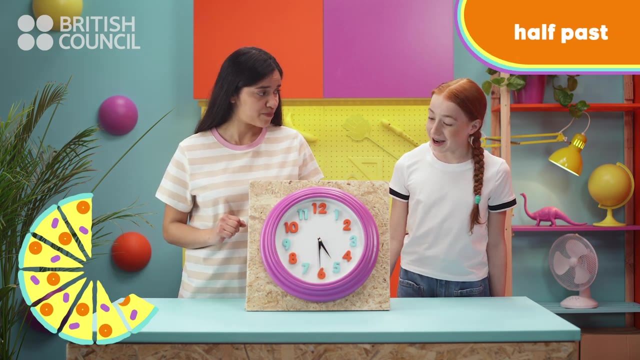 Because a quarter of the hour has passed. So what's the time Now? it's quarter past 5? Perfect. When the big hand is pointing to the 6,, we say it's half past Because half of the hour has passed. 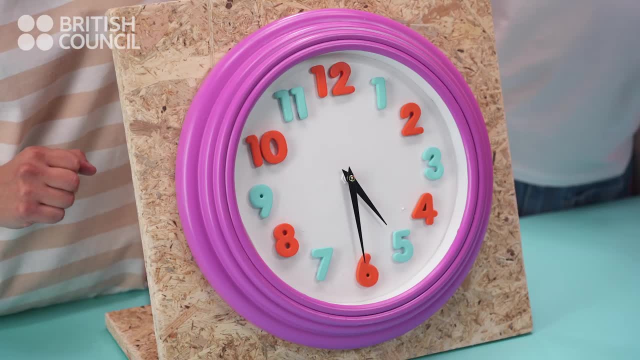 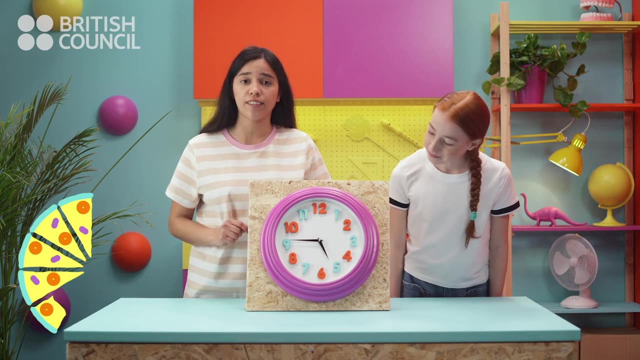 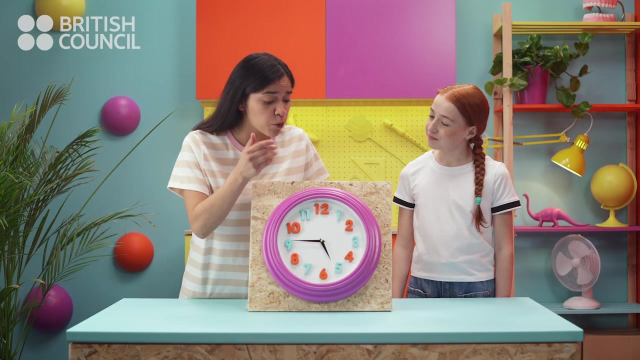 So now it's half past 5.. Fantastic. And finally, when the big hand is on the 9,, we say it's quarter to. So now it's quarter to 6.. Perfect. But what happens when the big hand isn't on the 12,, the 3,, the 6, or the 9?? 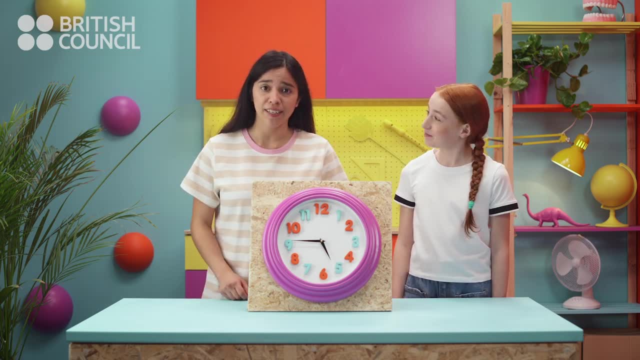 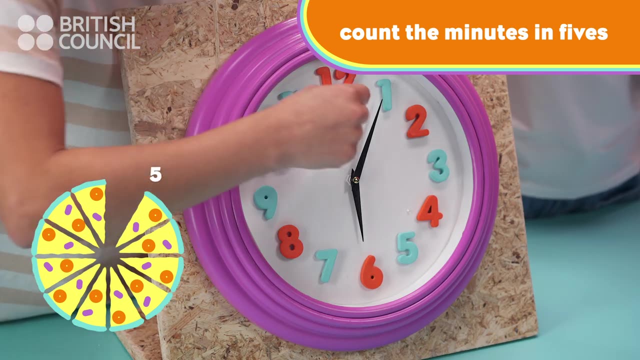 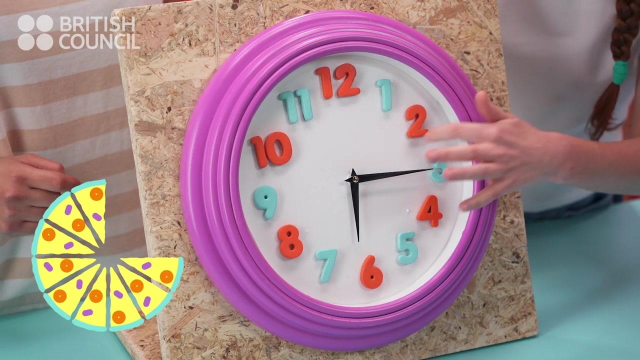 I don't know Well, we count the minutes in fives. So Now it's 5 past 6.. It's 10 past 6.. It's quarter past 6.. It's 20 past 6.. It's 25 past 6.. 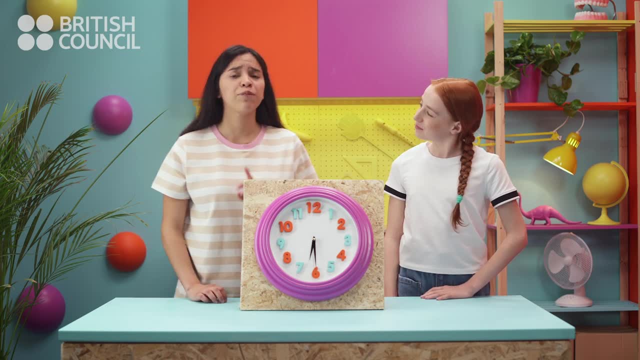 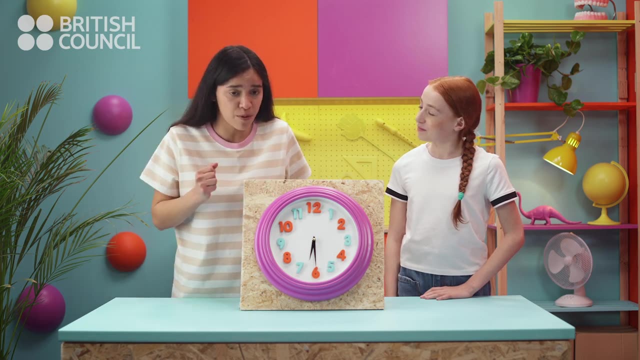 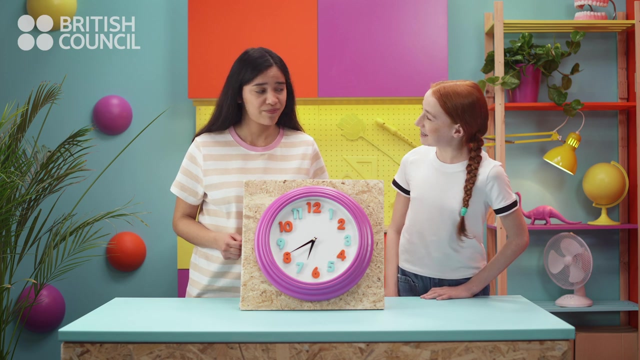 It's half past 6.. Wait a minute After half past it changes. Then we count how many minutes there are before the next hour. Remember it's 25 to 7.. It's 20 to 7.. I see. 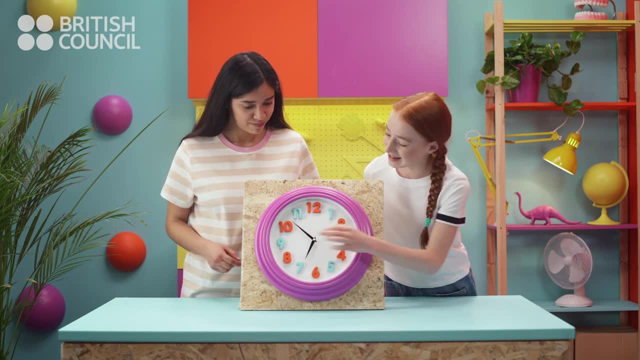 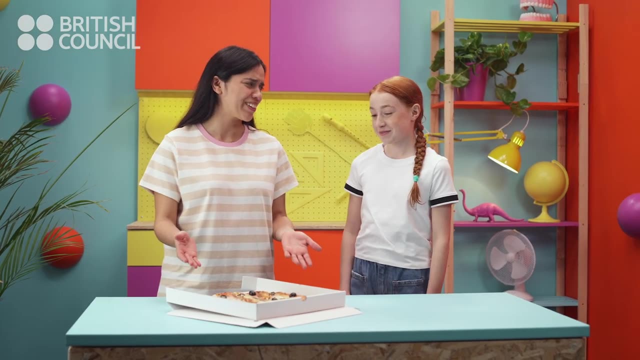 It's quarter to 7.. It's 10 to 7.. That's right. What time is it? I'm hungry. It's pizza o'clock. Yes, We hope you have fun learning to tell the time with us. Goodbye. 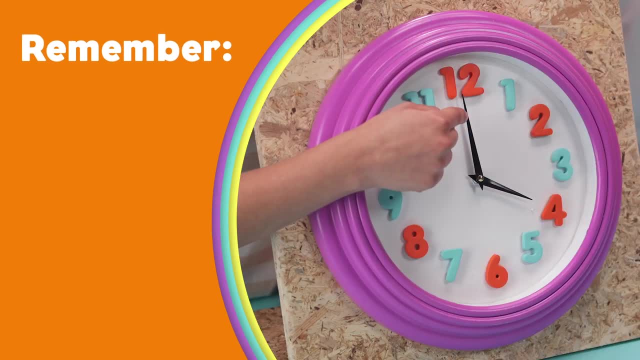 Remember to tell the time. When the big hand is pointing to the 6,, we say it's half past 6.. When the big hand is on the 12,, we say it's o'clock. When the big hand is on the 3,, we say it's quarter past.